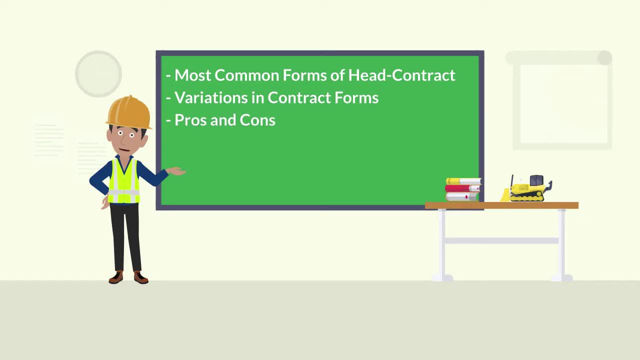 client and a head contractor. We talk about how these different forms vary and the pros and cons of each. If you find this video interesting and useful, check out the link in the description In the below description to our complete Udemy course on construction contract management. 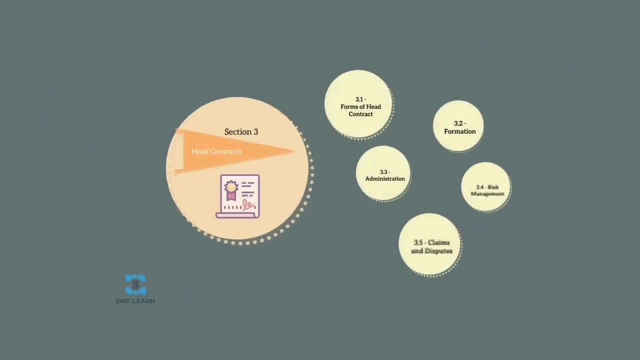 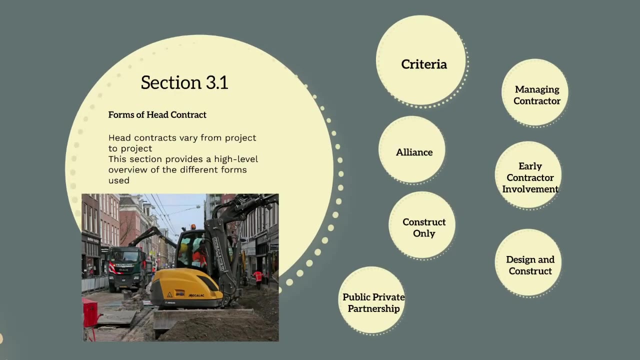 Hi and welcome to the first topic, first section of topic three, section 3.1, where we're going to talk about all the different forms of head contract. Head contracts vary from project to project and this section provides a high level overview of the different forms of contract that. 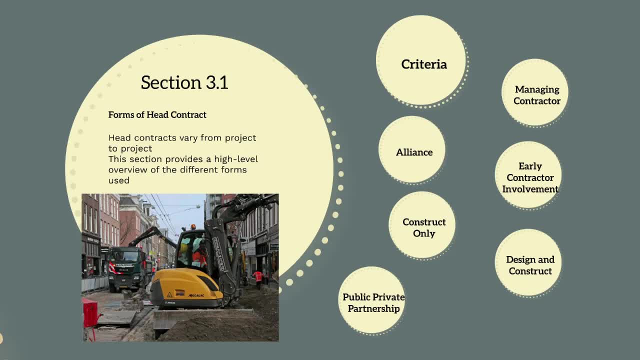 a client or project developer will use to engage a contractor. We're going to cover the criteria that head contracts vary around, followed by going through the most common form of head contract, including managing contractor, alliance, early contractor, involvement, construct only, design and construct, and public private partnership In each section. 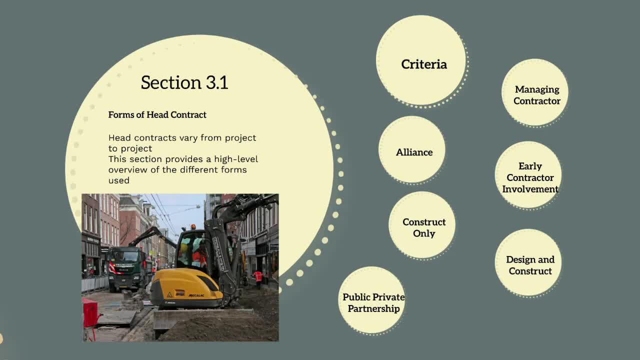 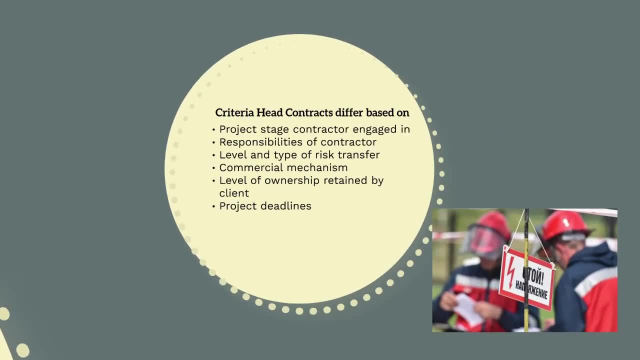 we'll go through the contract model and the pros and cons of that specific model. So what are the criteria around which different forms of head contract vary? Well, some of the key criteria with each form of head contract are the project stage during which the client will engage. 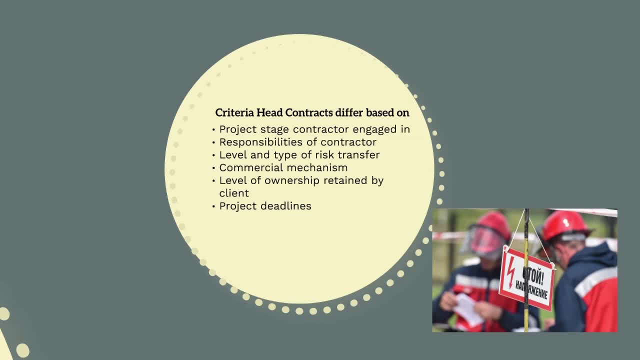 the contractor. so whether the client engages the contractor to get their involvement of them to manage the design or when the design is fully complete. the specific responsibilities of the contractor. the level of risk transfer and the type of risk transfer. so how much risk is the contractor exposed to. The commercial payment mechanism, so how the contractor gets paid. 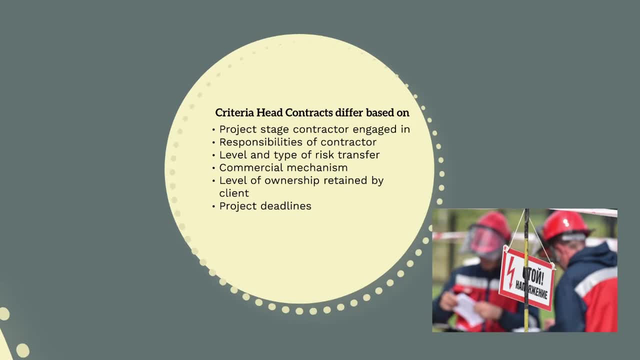 cost, plus the level of ownership and management retained by the client, and the project deadlines and specific project timeframe. Keep in mind, when we are going through the head contract forms, that the form of head contract will need to be adapted to suit the project, not the other way around. 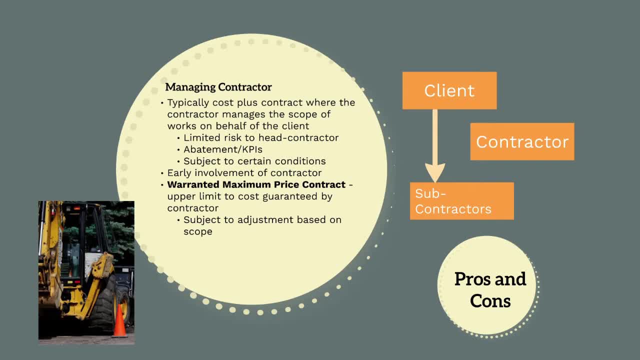 The first contract form we'll look at is the managing contractor model. This is where the contractor is engaged by the principal to manage the scope of works on behalf of the client. So if you look at the diagram on the right hand side, the client will be engaging the 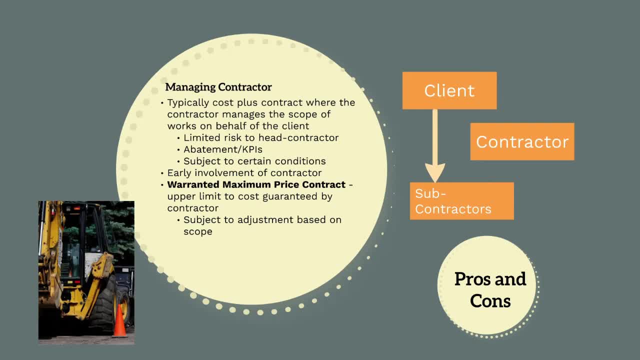 subcontractors directly. however, this process will be managed by the contractor. The payment mechanism is typically cost plus, with limited risk, passed on to the head contractor. However, the contractor may have abatements and KPIs depending on the performance of the contractor. 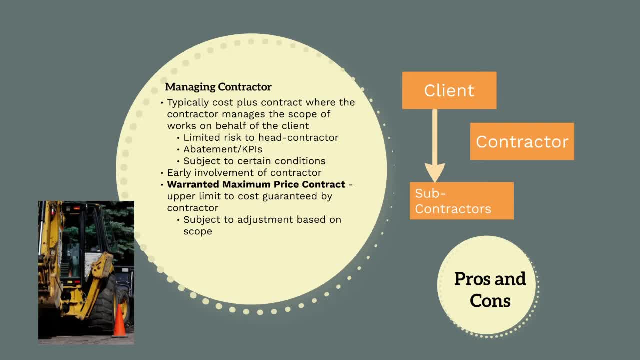 Additionally, there may be a warranted maximum price contract under which the contractor guarantees a maximum price for completing the works. Over and above this maximum price, the contractor will have to weigh the costs. Under a managing contractor model, the contractor will generally be engaged to provide input. 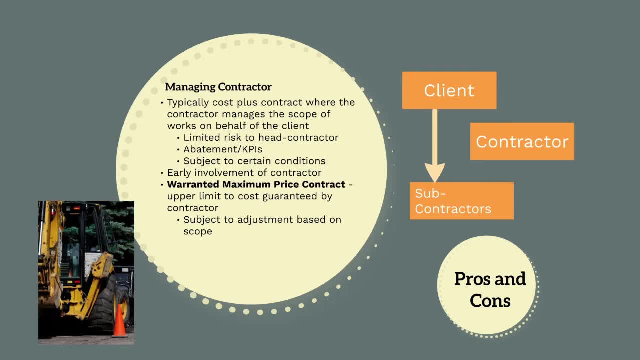 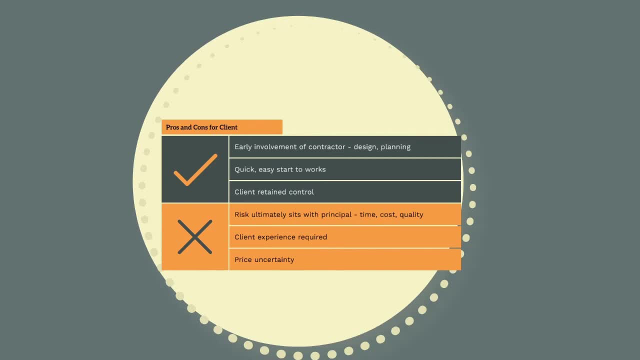 into the early project planning and design stages. One of the benefits of a managing contractor model from the perspective of the client is that the contractor is involved early, providing constructability, input and perspective into the design and planning. This may be expertise that the client critically needs but does not have. 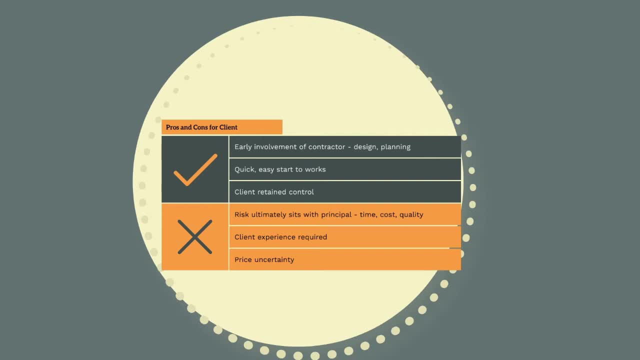 Furthermore, it's quick and easy to start works under this model. There is no need to map out a detailed scope of works and ensure all the risk is transferred to the contractor. Finally, the client needs to know how to manage the contract. This is where the contractor is involved early, providing constructability, input and perspective. 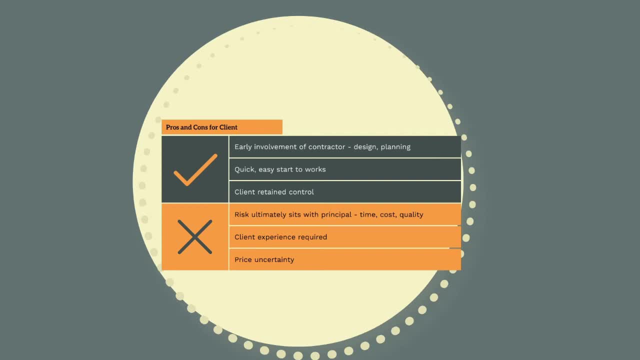 into the design stages. The client retains a lot of control over the works and can make decisions to influence them during the project delivery. Some of the disadvantages of this model is that the risk for time, cost and quality ultimately sits with the principal. They have not transferred this risk to the contractor. 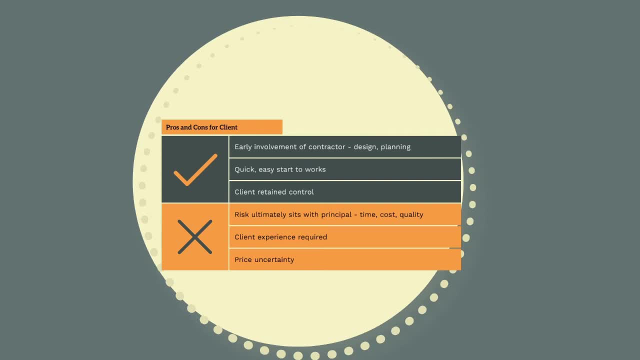 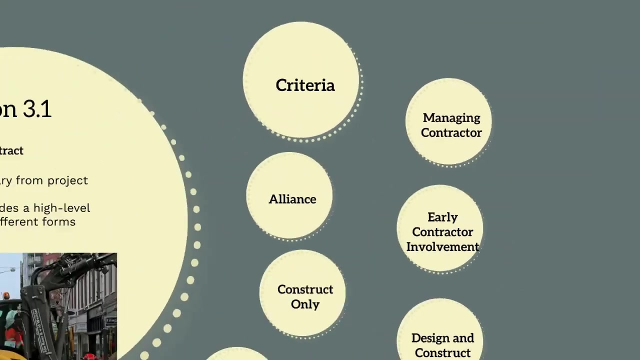 Additionally, a lot of client experience is required if they want to benefit from retaining control. Additionally, there is still a lot of price uncertainty. This can affect the client's financing of the project. The next model we'll look at is the alliance model. 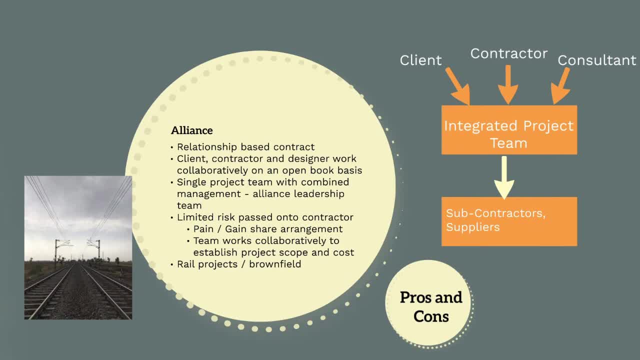 An alliance model is referred to as a relationship-based contract. The client, the contractor and the designer work collaboratively on an open-book basis to complete the project. They form an integrated project team from which they engage the subcontractors and suppliers necessary to complete the project. 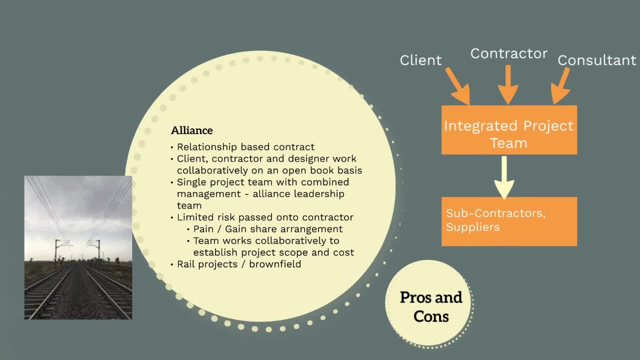 An alliance leadership team will be formed from all the members of the alliance that oversee the delivery of the project. Under an alliance contract, limited risk is passed on to the contractor. There is typically a paying or gain-share payment mechanism between the client and the 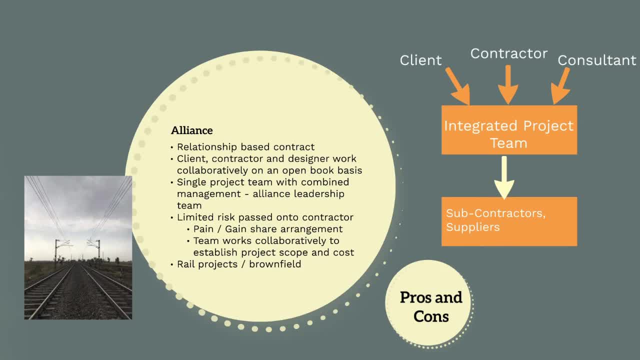 contractor, where the client and the contractor share in both profit and losses. The alliance team is generally formed at the project concept stage and the team will work collaboratively to establish the project scope and cost. Alliance projects are used typically when the project scope is not clear and extensive. 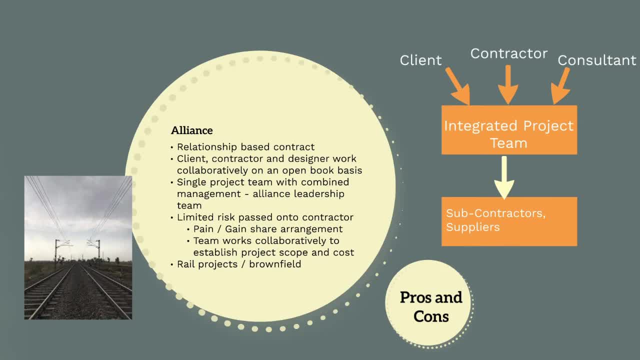 risks are involved. Forming the project team early and working together to form the project budget and schedule allows these risks to be transferred, understood, shared and managed effectively. Typically, alliance projects are used in rail environments, which are heavy brownfield environments with significant risks that can't be undone. 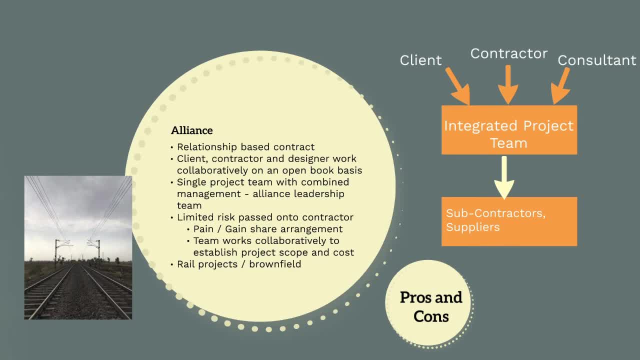 The alliance team is typically used when the project scope is not clear and extensive risks are involved. 고� pencils이DB-T기- Proscto-Trucks are used in rail environments where existing infrastructure is being upgraded and therefore the works involve impacting existing infrastructure. 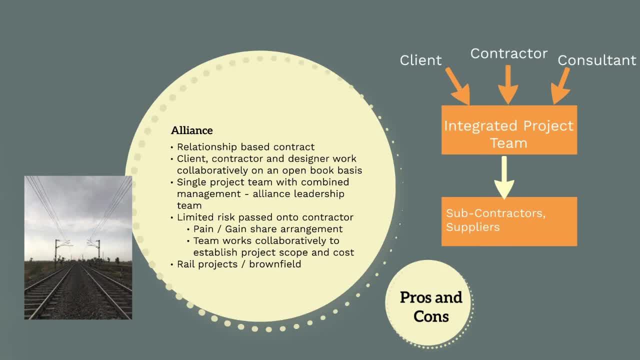 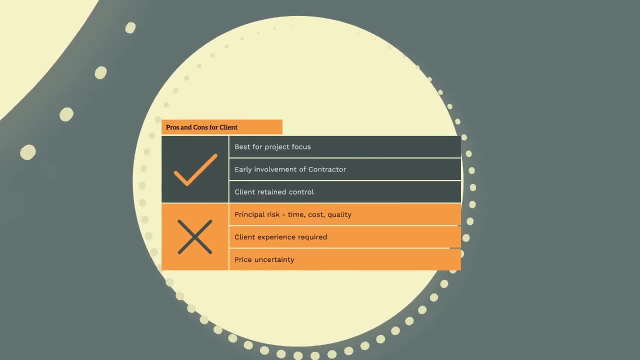 that might not be known or fully understood. This is opposite to a greenfield project: creating green infrastructure, which involves creating new infrastructure, especially when you have existing infrastructureovers, and Marsард infrastructure, Where an alliance contract works well, is to Establish the Best Project Focus for the Contractor. 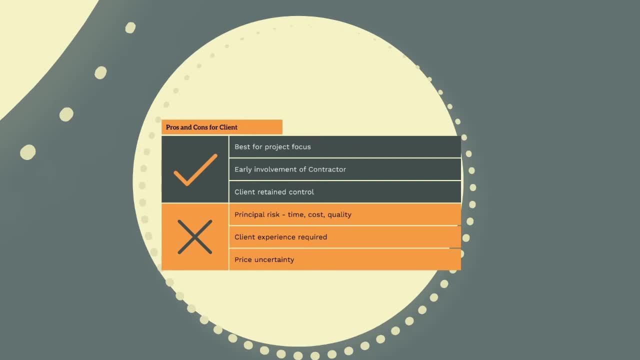 Additionally Dana-Ona Jesus, providing that the contractor is fully focused and most 风wheelsent. the contractor is responsible for the joint development of the project. in the project, sometimes one-to-one is involved at an early stage to maximise their input into the design and planning. 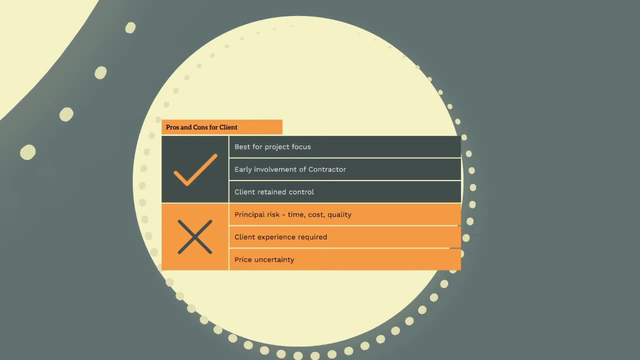 Furthermore, the client retains extensive control and has capability to implement and manage change. Again similar to a managing contractor model, the client still retains a lot of the project risks, as they are not transferred to a contractor. A more experienced client is also required to effectively control and make best-for-project. 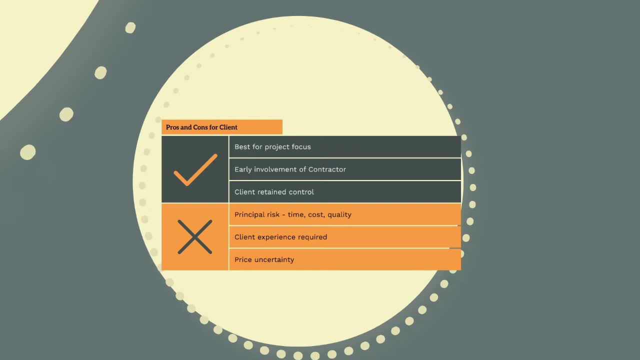 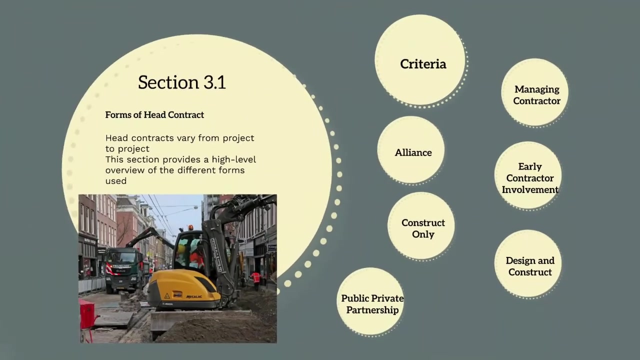 decisions. And finally, there is price uncertainty, as a lump-sum price has not been passed on to the contractor. This may make the project feasibility analysis harder for the client, as total costs are more uncertain. Under an early contractor involvement or ACI model, the contractor is engaged early. 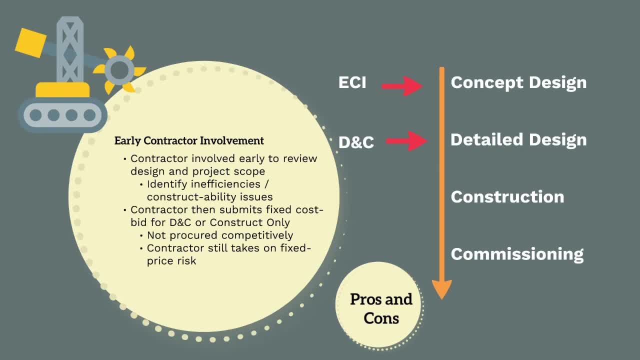 to review the design and project scope. This is done to identify inefficiencies and provide constructability input into the design process. The contractor is generally engaged prior to the concept design stage, as opposed to a typical design and construct contract, where the contractor is engaged to complete the 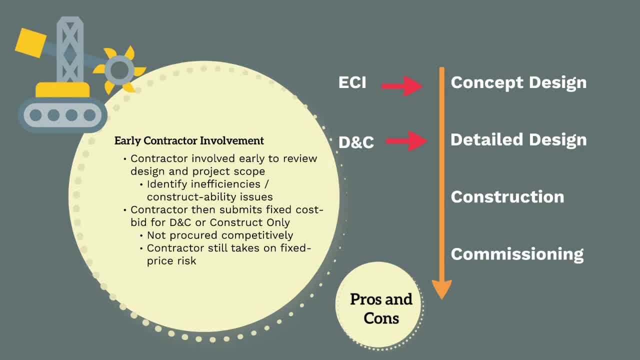 detailed design and construction. Once the contractor is provided input into the design and development and project planning, the contractor will then submit a fixed cost for the complete design and construction or construct-only scope. Under this second stage of bidding, the works are not procured competitively, but the contractor 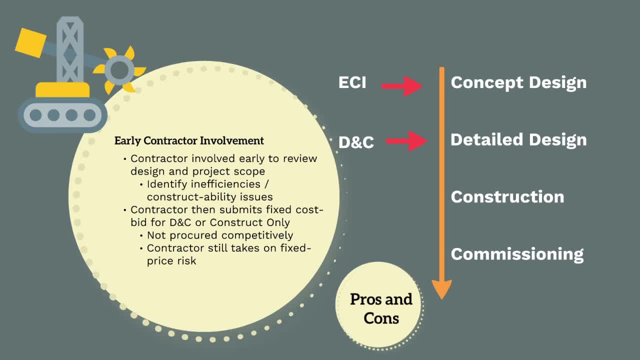 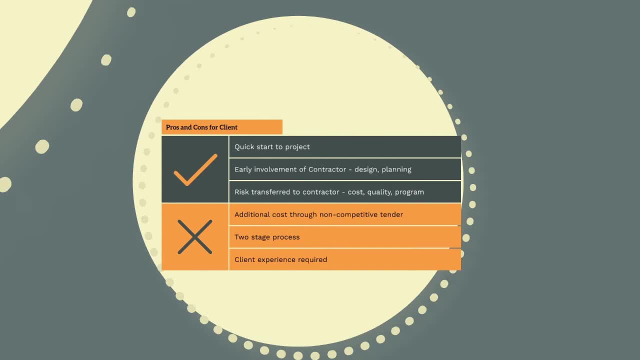 will take on the risk of completing the works to a fixed lump-sum price. The pros of an ACI model are that there is a quick start to the project. The contractor is engaged early with limited risk to support the design and detailed planning. 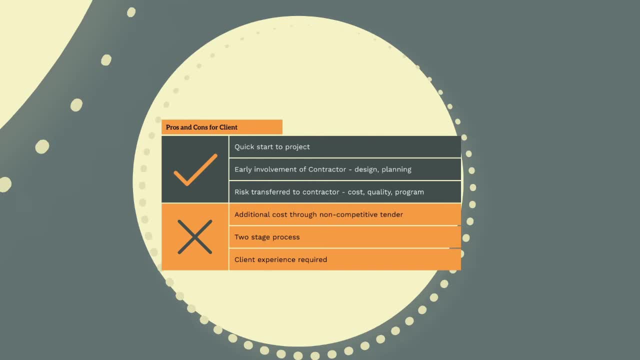 The input is a major advantage, as well as the constructability. reviews to the original planning and design will often prove invaluable once construction begins. Another advantage of an ACI model is that after the initial bidding, the contractor submits a fixed price for the works. 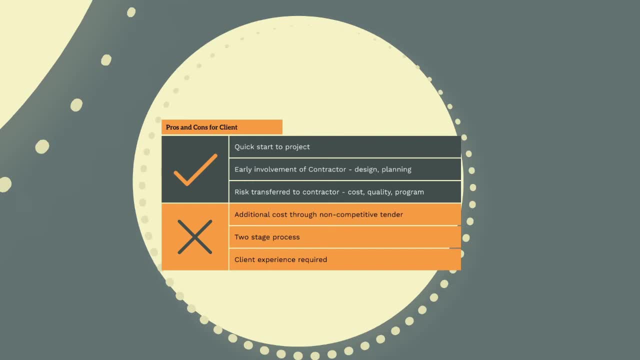 The ultimate project risk for cost, quality and program is transferred to the contractor. Some of the disadvantages of an ACI model from the perspective of the client is that the contractor is procured under a non-competitive tender, meaning they may increase their prices. 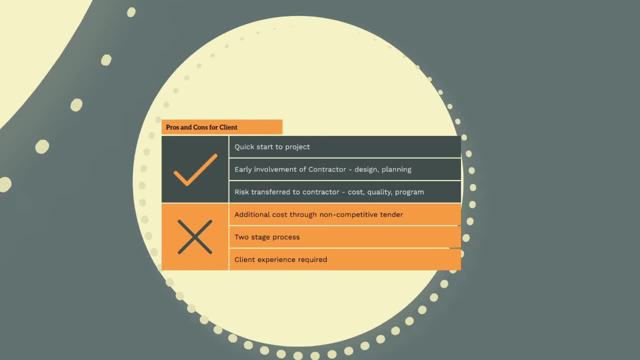 as they know, they're not having to beat competition from other contractors. This is different from a DNC model where there is competition between the contractor and between potential contractors. Furthermore, the ACI model requires a two-stage process which can add time to the overall. 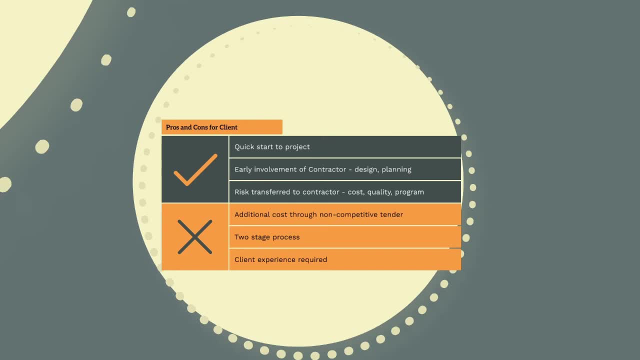 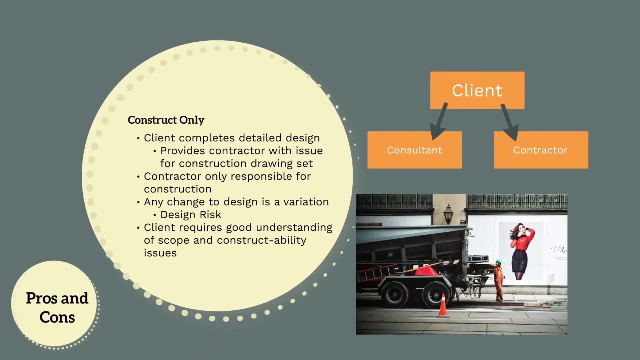 project schedule. The contractor will need to prepare and submit a fixed price quote after the design stage. Furthermore, client experience is required to ensure that the DNC scope can effectively be managed Under a construct-only scope. the client completes the detailed design and issues the contractor. 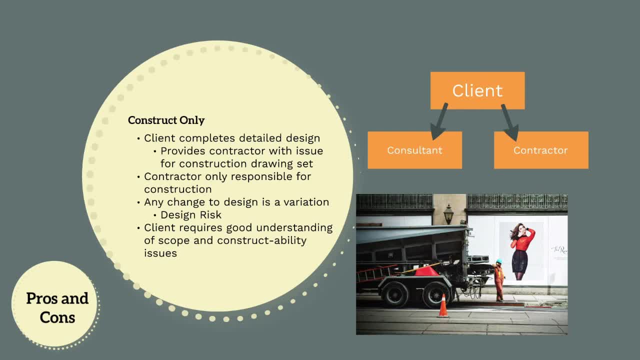 an issue for construction. The client is responsible for completing the design and any changes to the design would constitute a variation to the project scope. The contractor is only responsible for the construction. To complete this, the client will need a good understanding of the project scope and be 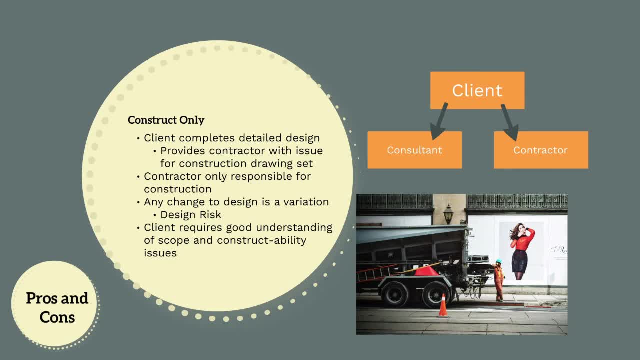 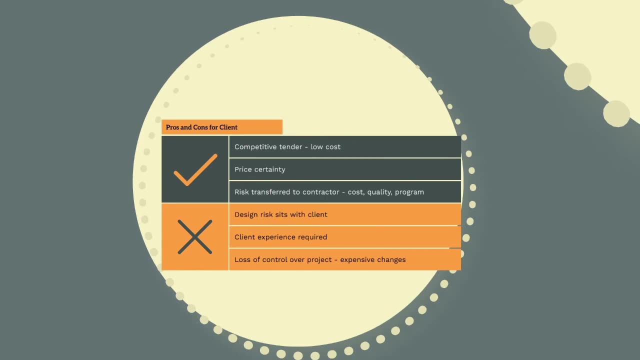 able to resolve any constructability issues with the design. We can see this structure in the design on the right, where the client procures both the consultant and the contractor. Some of the advantages of a construct-only package from the perspective of the client is that the procurement of the contractor is run through a competitive tender meaning. 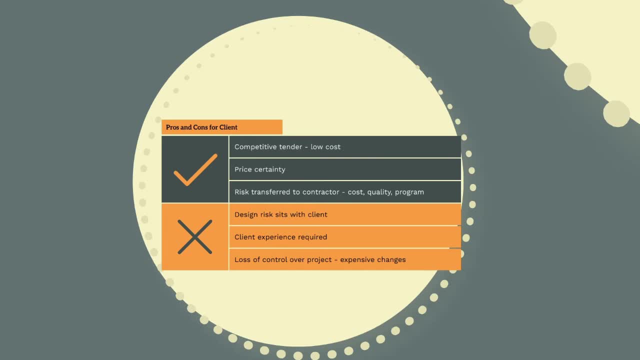 there is price competition between contractors. Contractors will bid for the works with lower profit margins and less contingency to ensure they win the project. Furthermore, the client will have price certainty, meaning they know how much the project will cost, based on the contractor's lump sum price. 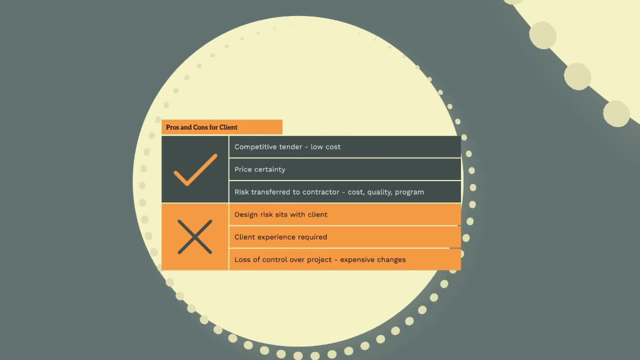 The contractor will be able to determine the cost of the project based on the contractor's lump sum price. The contractor will have the right to decide the cost of the project based on the contractor's lump sum price. The contractor will be able to determine the cost of the project based on the contractor's 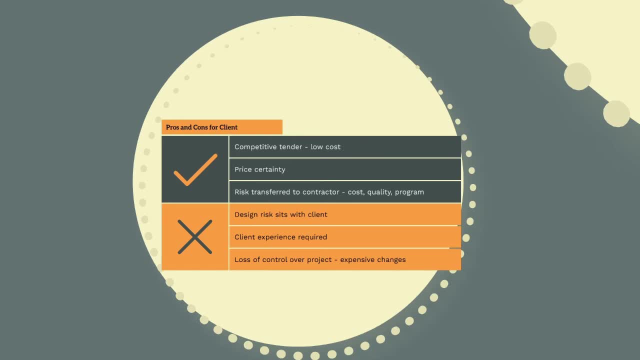 lump sum price. Finally, risk is transferred to the contractor to manage. They are responsible for managing costs, quality and the project schedule. Some of the disadvantages of a construct-only contract model is that the design risk sits with the client. They are responsible for reducing the design and any inaccuracies, errors or omissions. 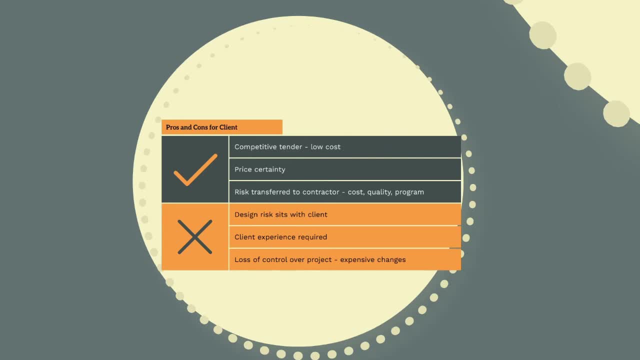 in the design will result in expensive rework and variation from the contractor. The client experience is required to make sure the design is completed correctly and any constructability issues are identified and resolved. Furthermore, once the contract is awarded, the client effectively loses control over 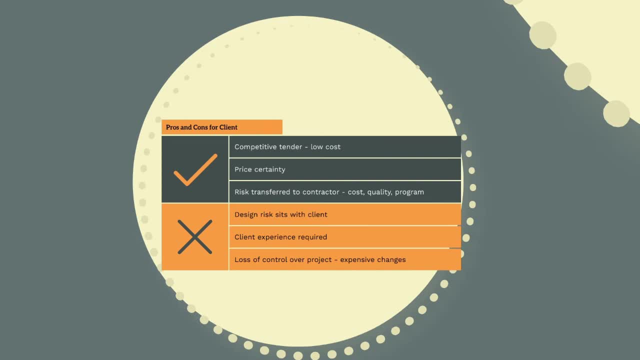 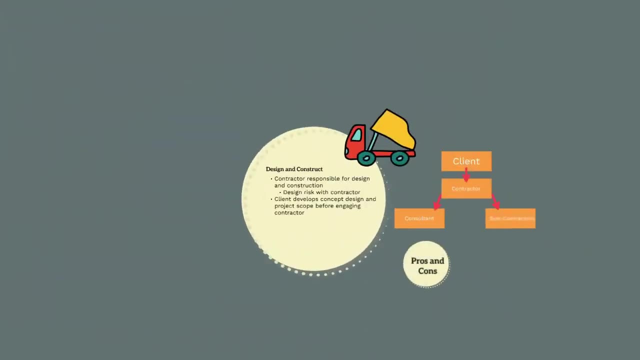 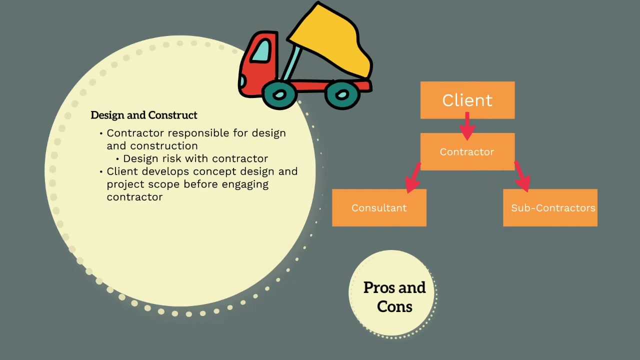 the project. If the client wishes to change the scope, they will need to pay expensive variations to change things. A design and construct or DNC project is the same as a construct only contract, except that the contractor is also responsible for the development of the detailed design. 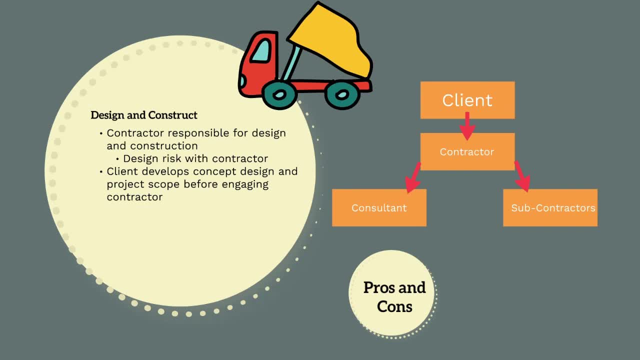 Therefore, the design risk has been passed on to the contractor. The client will need to procure a concept design showing roughly what they want and project scope. The contractor will then base their quote to take this concept design, produce an issue for construction design and then build it. 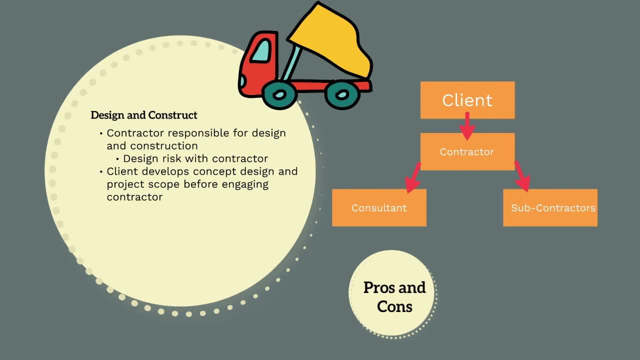 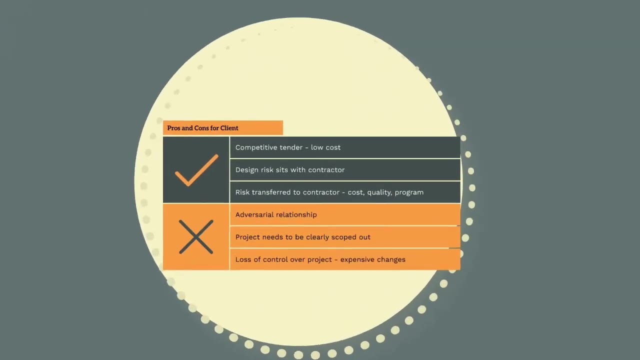 You can see this set up on the diagram to the right where the contractor is engaging both the consultant to complete the design. Again similar to a construct only contract. a DNC contract will have a lump sum payment mechanism. Similar to a construct only contract. the pros and cons from the perspective of the 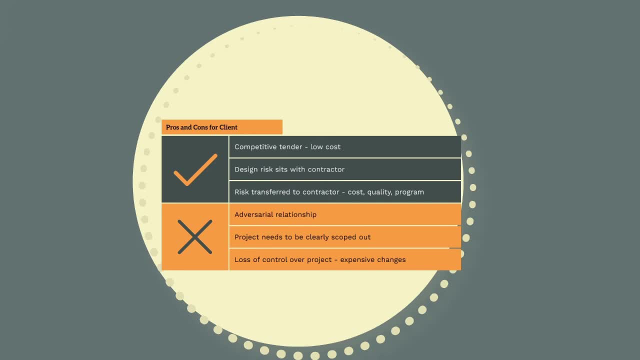 client. a DNC contract will result in price competition between potential contractors, resulting in a lower price for the client. Contractors will cut risk contingency. The contractor will be responsible for managing the design risk and profit margins to secure the project. Furthermore, under a DNC, the contractor is responsible for managing the design risk. 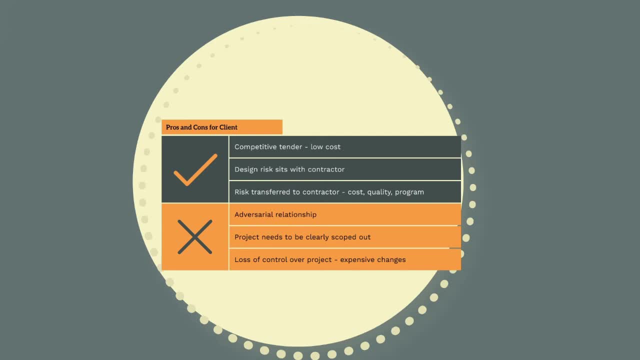 and this is often a significant project risk. Again, under a DNC, most risks are transferred to the contractor, who is responsible ultimately for cost, quality and program. Some of the disadvantages of a DNC model from the perspective of the client is that it can: 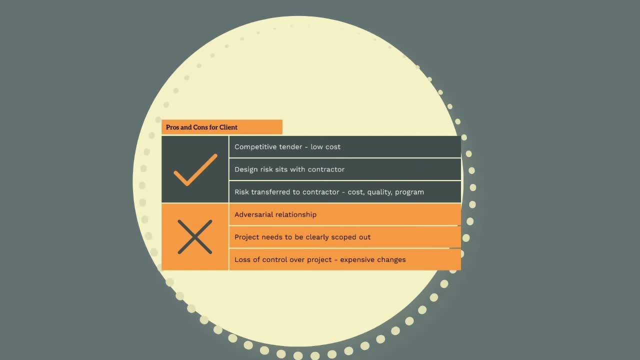 result in adversarial relationships between the contractor and the client. The client will be responsible for managing the design risk and this is often a significant project risk. The contractor may be exposed to extensive risk under low profit margins. There will likely be numerous disputes about cost and scope, particularly about the design. 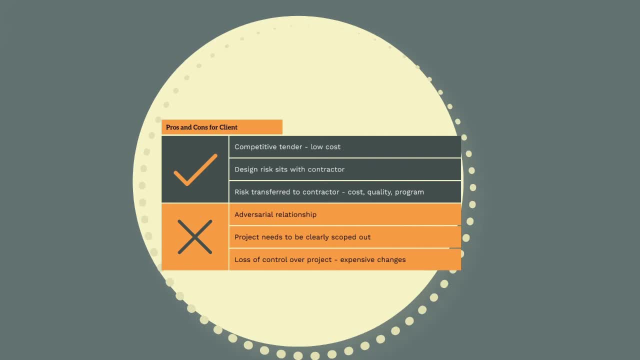 development and interpretation of the project requirements from the concept design. I've worked on a DNC project where requirements were murky and unclear, resulting in constant battles with the client. Furthermore, the project will need to be clearly scoped out and requirements for the contract are understood. 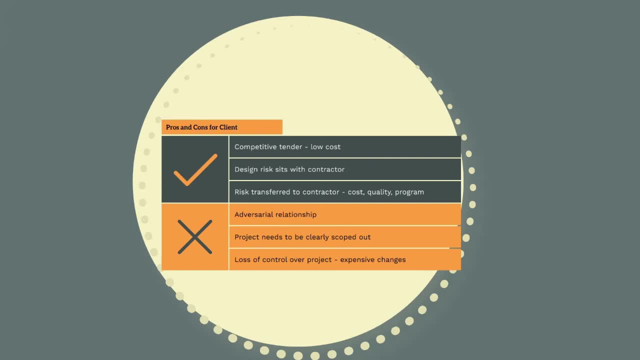 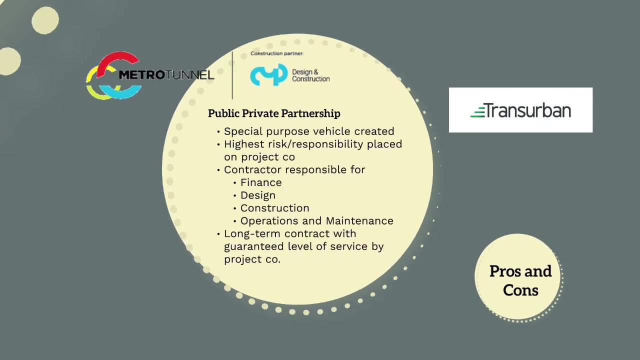 Again, the client will lose a lot of power to change things and once the works begin and the contract is awarded, any changes will need to be made through expensive change orders. A public-private partnership is the procurement model with the greatest risk and responsibility transferred to the contractor. 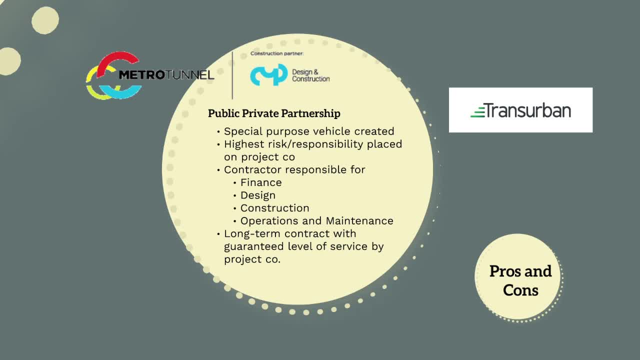 The contractor will generally form what's called a special purpose vehicle or consortium that, given the project, completes the finance, design, construction, operations and maintenance of the project. So the contractor will form a consortium with investment banks and operations and a maintenance provider to complete the entire project scope from start to finish, including the maintenance. 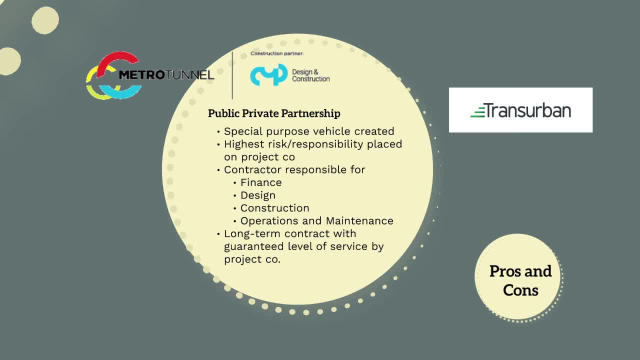 period. In this way, the client- typically government bodies, as PPPs are generally only used for massive multi-billion dollar projects- simply has to pay the consortium A fixed annuity over the project life, typically 25 years, and all the risk and responsibility. 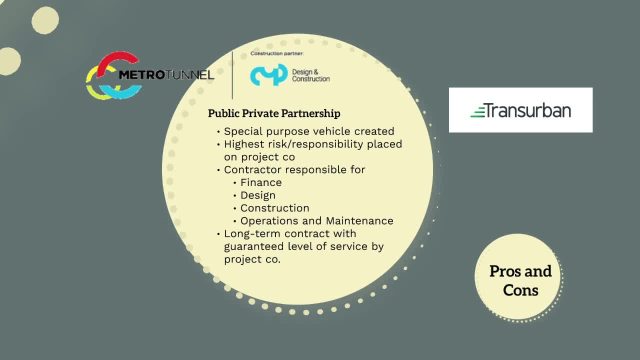 is on the consortium. This means the consortium will need to organise the financing of the project, take the concept, design and construct it in the most effective way, while also minimising the whole of life operations and maintenance cost. Some examples of PPP projects include the tunnel and stations package on the New Melbourne. 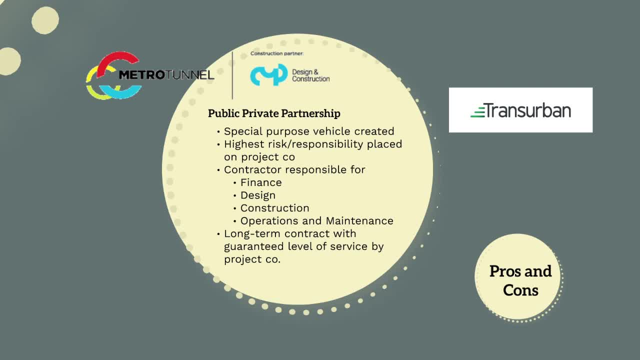 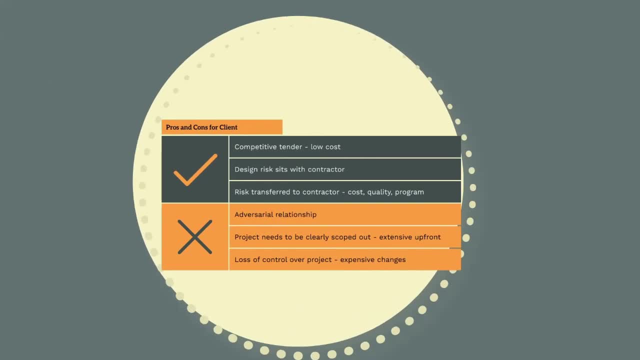 Metro, Tunnel And Transurban Building. Some of the advantages of a PPP model are that they are procured competitively, so potential contractors will have to competitively bid for this massive scale project. They will try to cut costs, and so the government should theoretically get the most cost competitive. 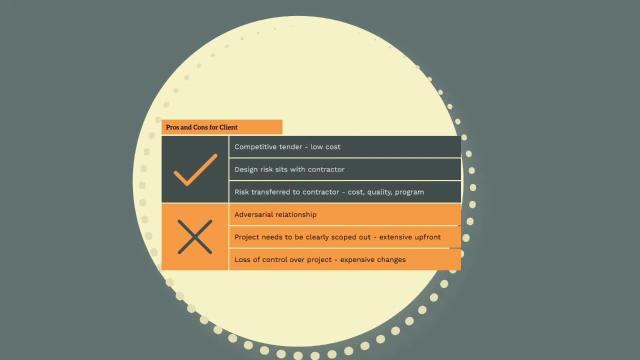 outcome. Furthermore, the design risk again sits with the contractor, but in this instance the contract needs to design something. The contract needs to design something that also has a whole lot of potential. The contract needs to design something that also has a whole lot of potential. 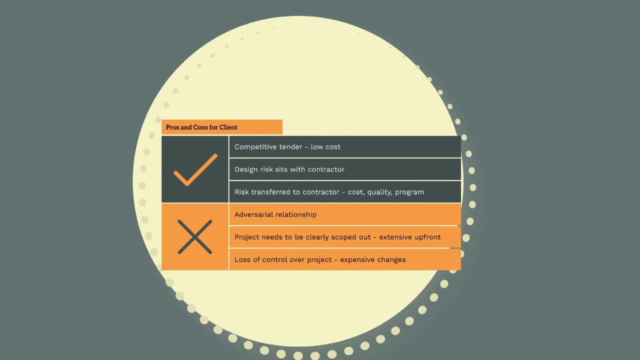 The contract needs to design something that also has a whole lot of potential. The contractor needs to design something that will have a reasonable low whole of life value. In this way, the contractor needs to factor in construction costs, maintenance costs and finance costs, and so, ideally, will bring all these components of the project together to 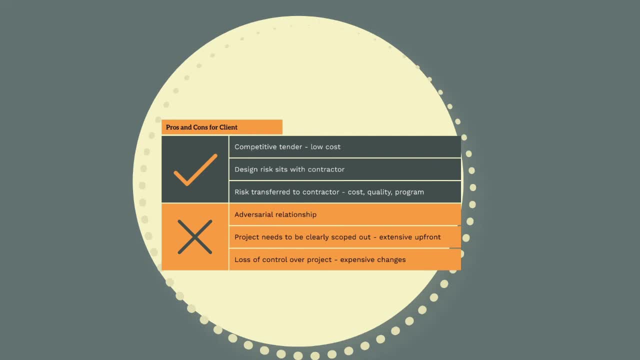 develop the best solution for the project. And finally, all risk is transferred to the contractor, not just the DNC Scope, but also the financing and maintenance risk. So what are the cons? Well, similar to D&C projects, PPPs lead to adversarial relationships between the contractor. 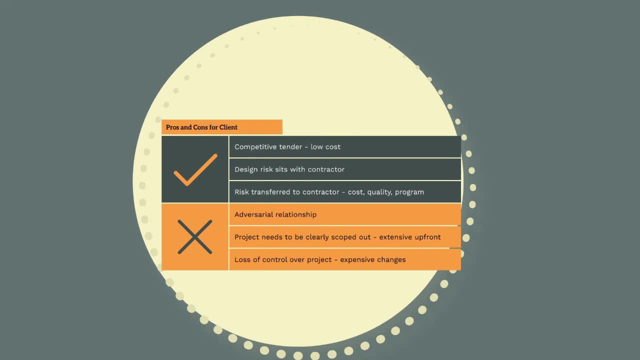 and the client. Most PPPs end up in some sort of dispute. A significant part of it is differing interpretations of scope and expectations. In addition, such a huge amount of risk is passed on to the contractor that there is a significant chance that the contractor does. 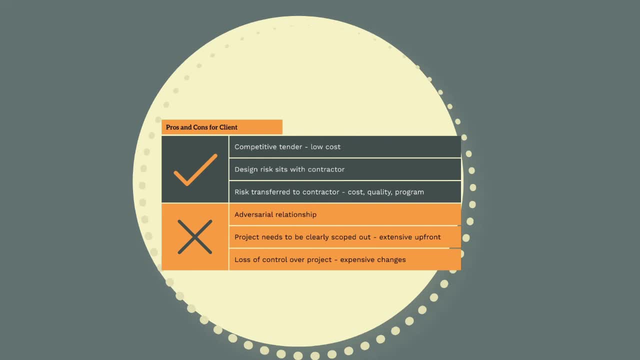 not have enough contingency factored in and may lose money completing such a project. This will likely be incredibly difficult and lead to extensive disputes and delays. Finally, the client will lose all control over the project. Variations under PPPs can be much more expensive than under D&C projects, as now the client when instigating changes.